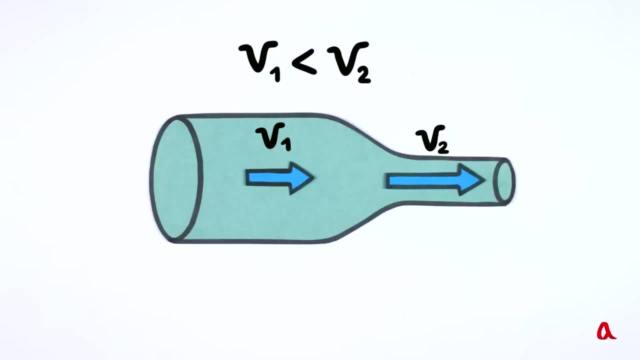 water flow increases. According to Newton's second law, in order to increase the speed, some force must be applied to water. Thus, the pressure in the wider part of the pipe must be higher than that in the narrow one. Therefore, when the pipe gets narrower, the pressure in it will not rise as it may seem at first. 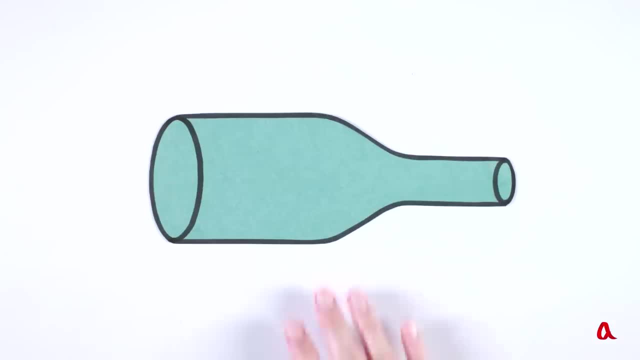 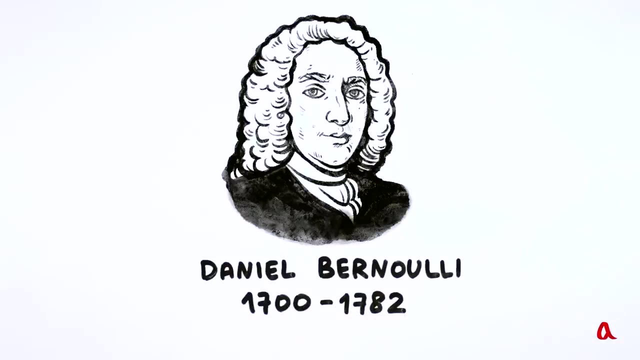 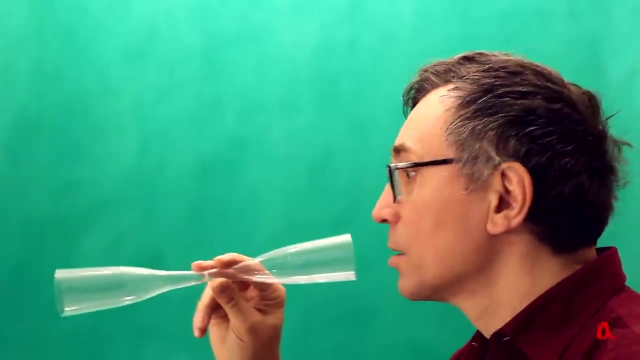 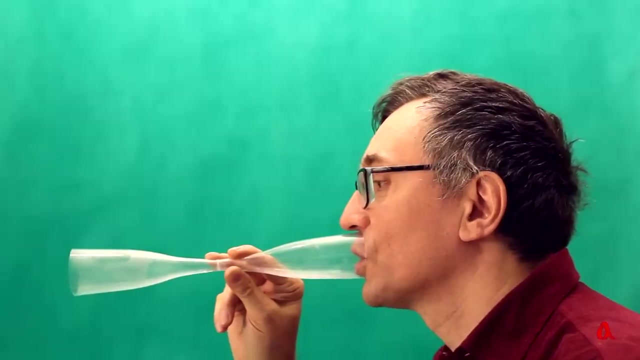 sight but fall. This puzzling paradox is called Bernoulli's principle in honor of its discoverer, a Swiss physicist, Daniel Bernoulli. We made this narrow neck pipe from two plastic glasses. When we blow it, the air pressure at the exit will be equal to the atmospheric one. This means that inside the narrow neck, 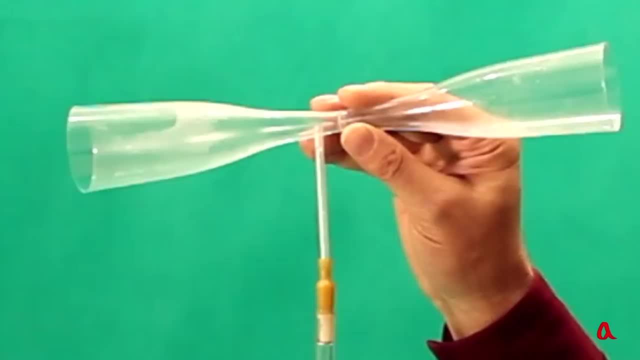 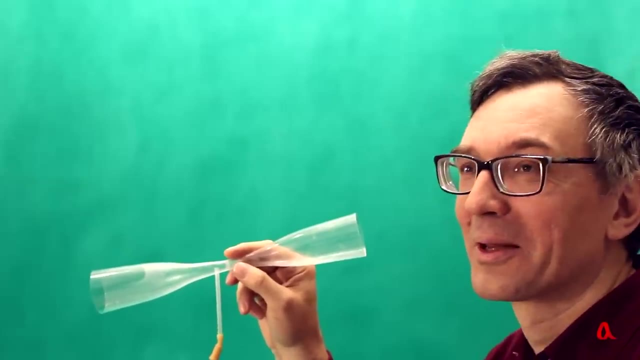 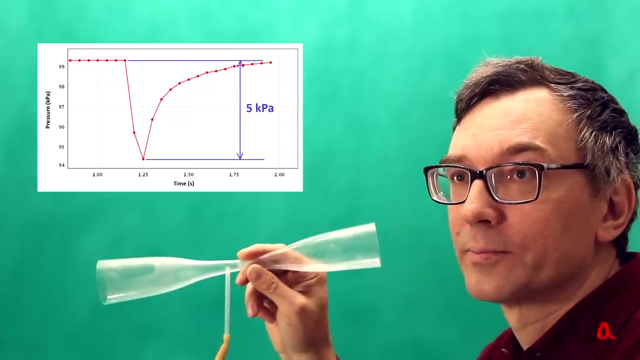 it will be lower than the atmospheric one. To check this, let us insert a tube into the wall of the neck, connecting it to a pressure sensor. When we blow the pipe, the sensor shows the decrease in pressure by 5 kPa, which is 50 cm of water column. 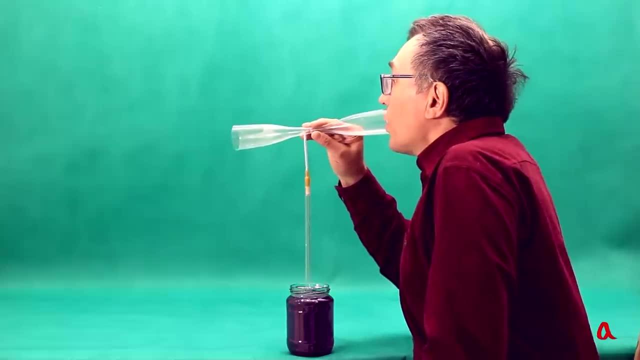 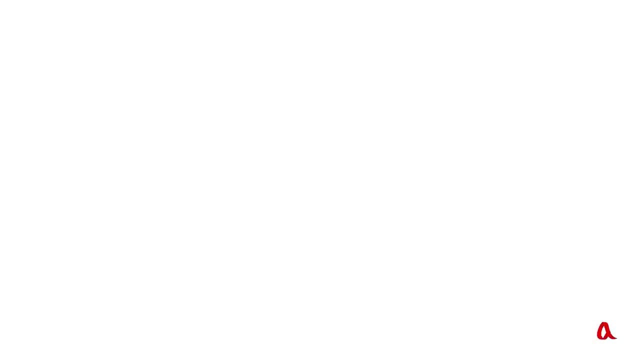 Let us put the lower end of the tube into the vessel with colored water and blow the pipe again. We can see that the water makes a 30 cm rise. To increase the pressure even greater, we'll connect the pipe to the blower, which provides a 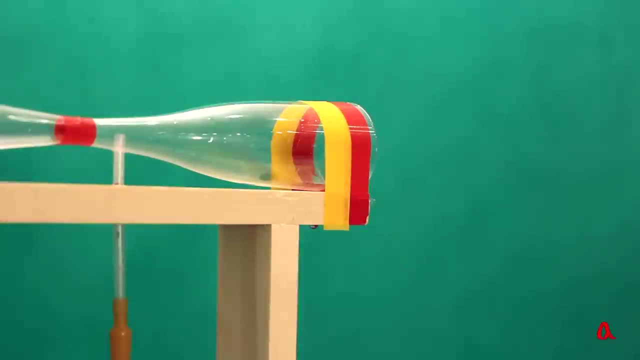 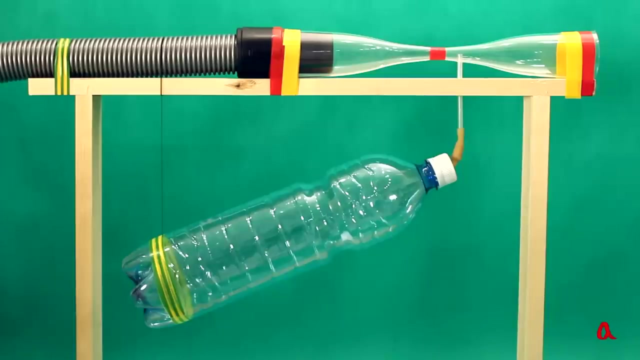 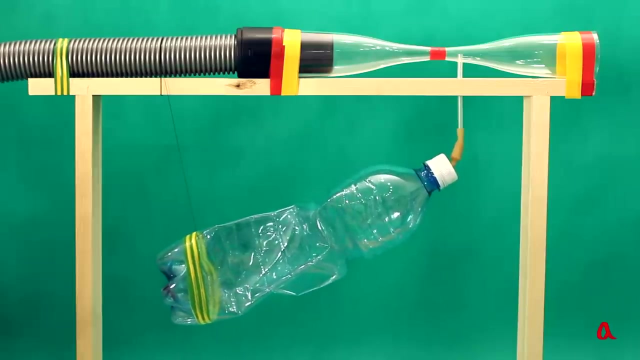 far higher speed of the airflow. We switch on the blower and what we get is a perfect water sprayer. Now let us attach a plastic bottle to the pipe and switch on the blower again. That's incredible. A decrease in the internal pressure causes the bottle to be crumpled. 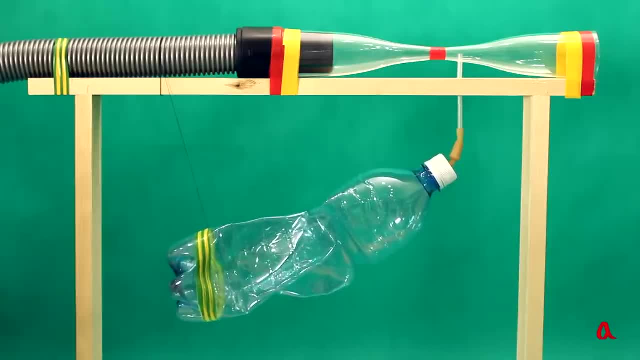 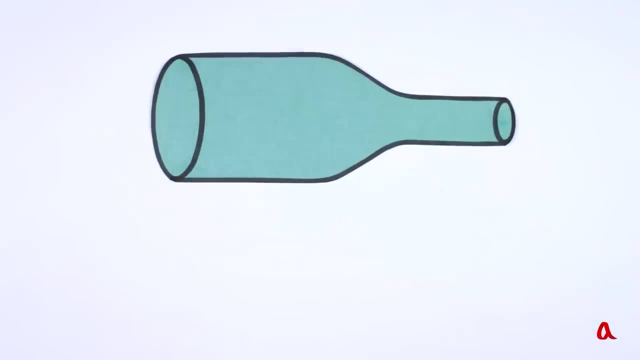 by the outer atmospheric pressure. Let us consider water flowing inside a cross section pipe. The volume of water V enters the pipe from the left end and leaves the pipe on its right end. The difference of pressures at the ends of the pipe does mechanical work, which equals P1 minus P2 multiplied by V, When